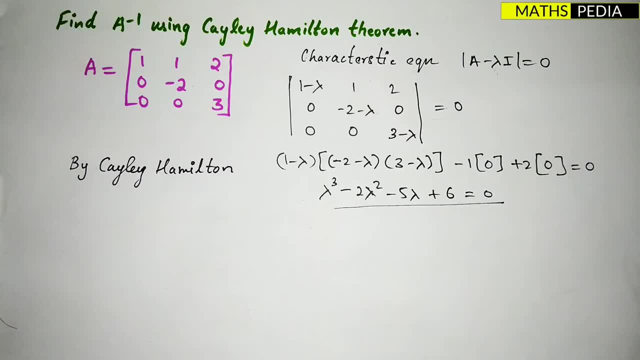 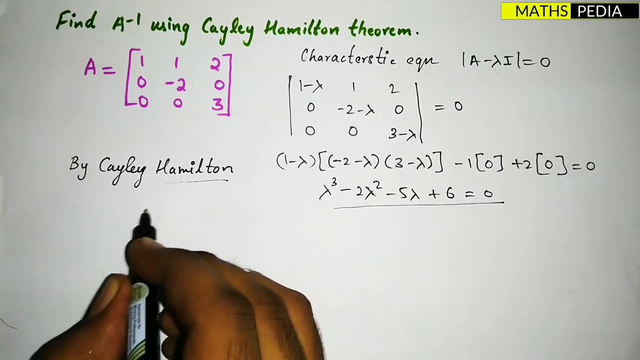 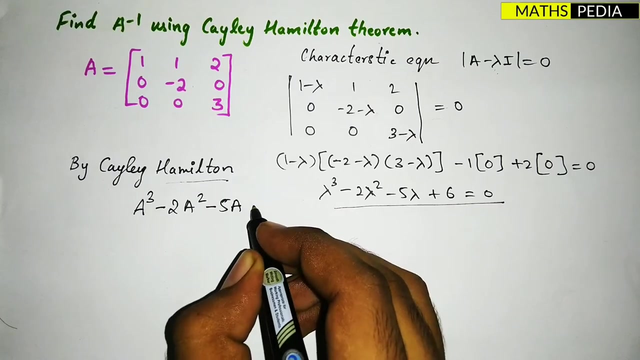 equation. this is the first step you need to do now. by Kelly Hamilton theorem we can say that, not it. every square matrix. every square matrix satisfies its own characteristic equation. that means I can replace the lambda with what, a? so it becomes a cube minus 2, a square minus 5, a plus 6 is a constant. since I want matrix of the, 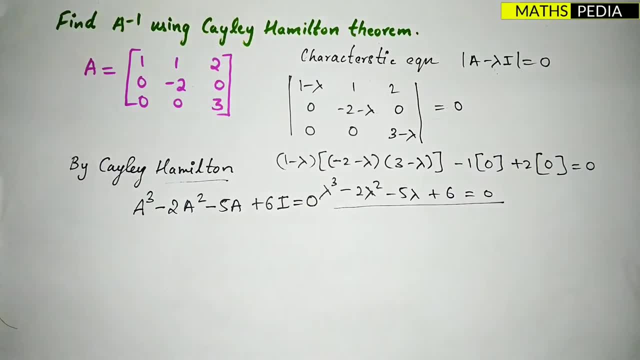 same order. I will replace with I, identity matrix. okay, simple, identity matrix. it will be order of what? 3 cross 3. only now we need we need to find the inverse of the given matrix. so I will just multiply with a inverse, so this equation becomes a inverse into a cube minus 2, into a square, into a inverse minus 5, into a into. 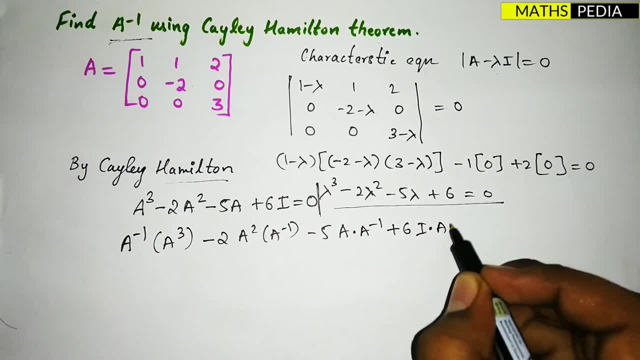 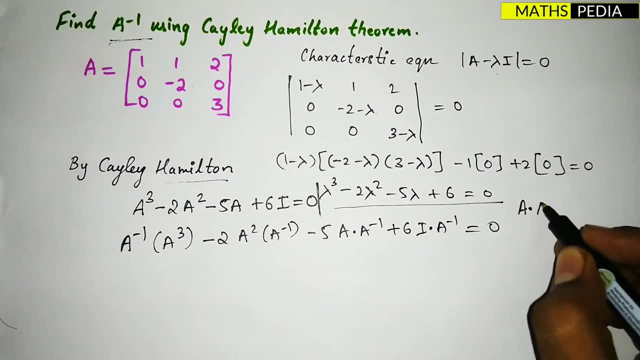 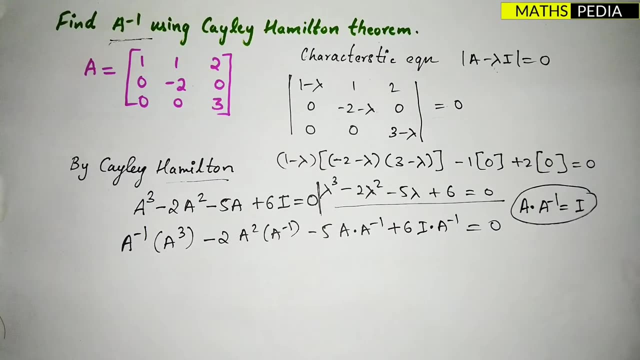 a inverse plus 6 into I into inverse, which is equal to 0. now, here you have to use the one property, that is a into a inverse is equal to what identity matrix? okay, a into a inverse is for identity matrix. so A inverse into a. this becomes. 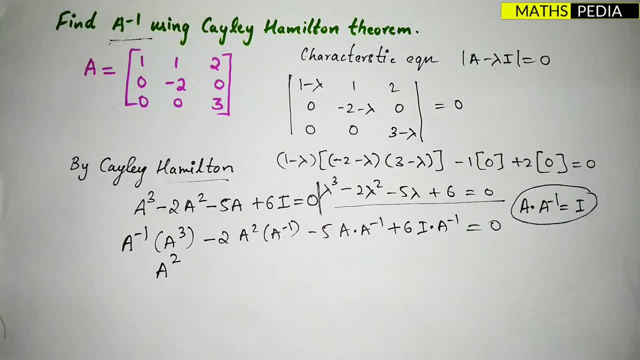 I write a square- okay, minus a square- into this thing. so 2a: just reduce one power, that's it. so minus a- into a inverse, that is, 5i plus 6i into. this becomes what 6a inverse i'm just using, just shifting it to other side. so you'll get the equation. okay, shift this to other side, you'll. 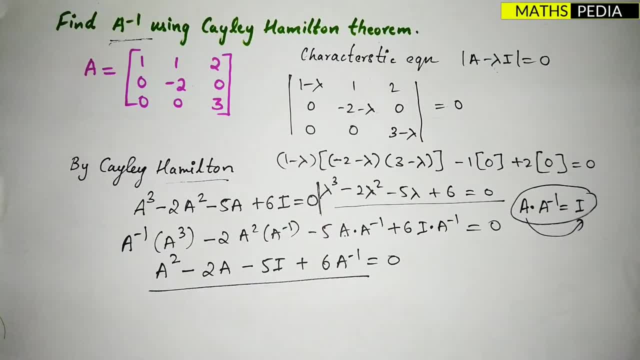 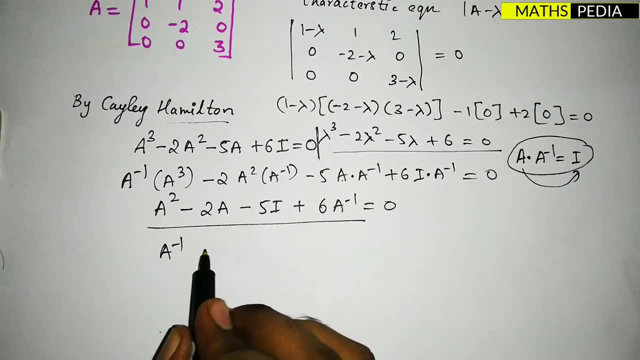 get this equation a inverse. now, here we have formed the equation, now you have to just solve this. so here keep a inverse. on one side, since we want to find, and others you have to just shift it off 1 by 6. okay, it becomes what 5i plus 2a minus a square. so you need to find a square also, so you 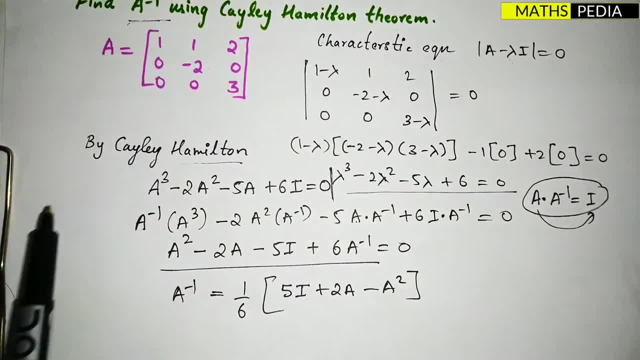 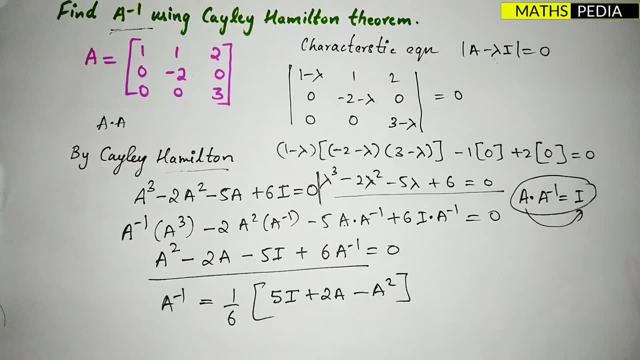 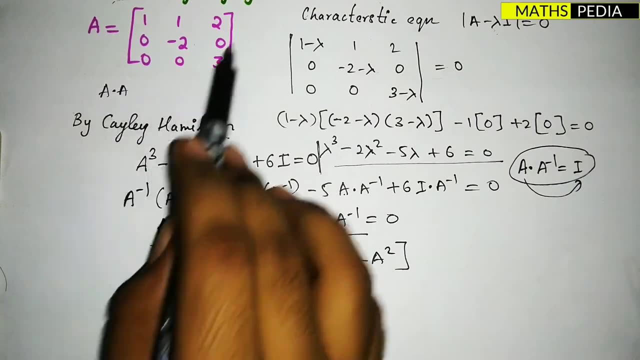 have to just multiply what this matrix twice. that means a into a. don't just square each element. okay, that is not the right way to do the multiplication of the same matrices or the other. we can say now: a square means a into a a you have to take one more.